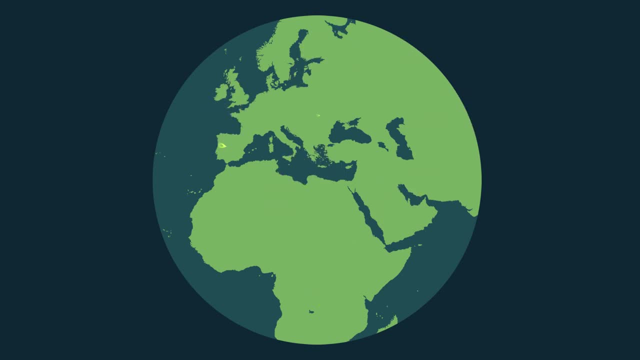 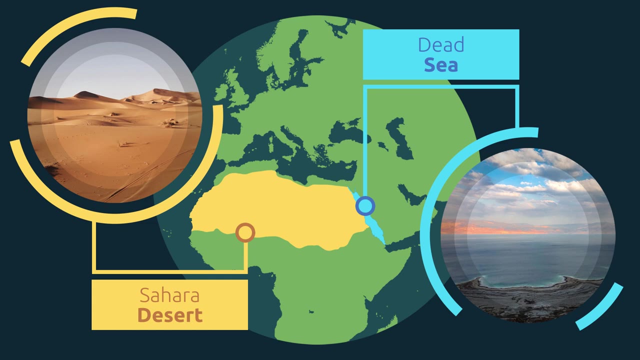 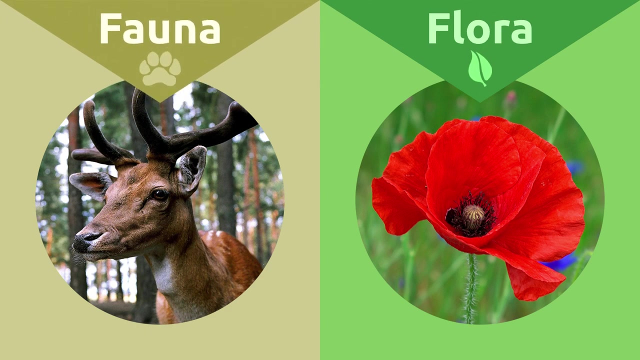 Ecosystems are found in different parts of the planet. They can be very big, like the Sahara Desert, or much smaller and circumscribed, like the Dead Sea. But how do we identify ecosystem coverage? The flora and fauna of each ecosystem have adapted to live according to the characteristics. 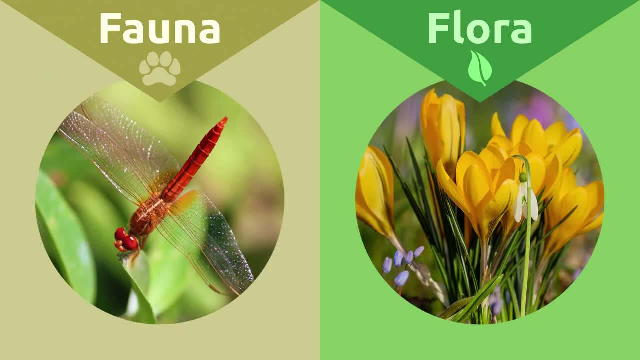 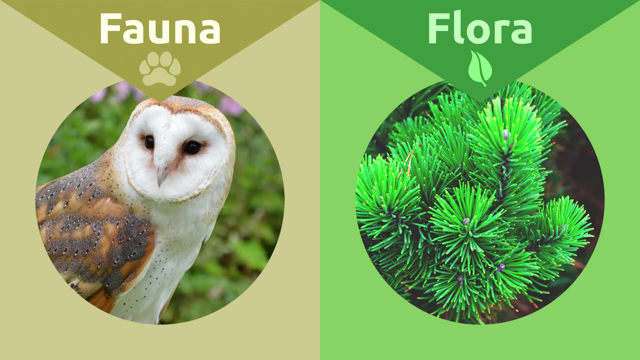 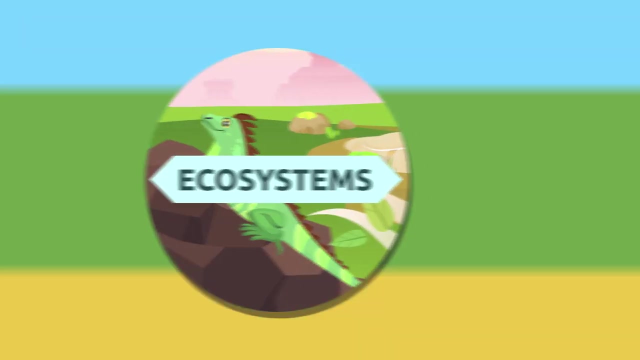 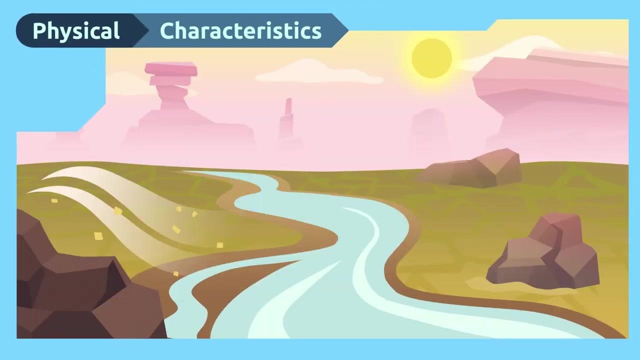 and resources of their surroundings. The interaction among them defines the ecosystem and its coverage. That's why there are so many types of ecosystems. Ecosystems consist of a biotope and a biosynosis. Let's see what they are. The physical characteristics of the surroundings are called a biotope. These characteristics 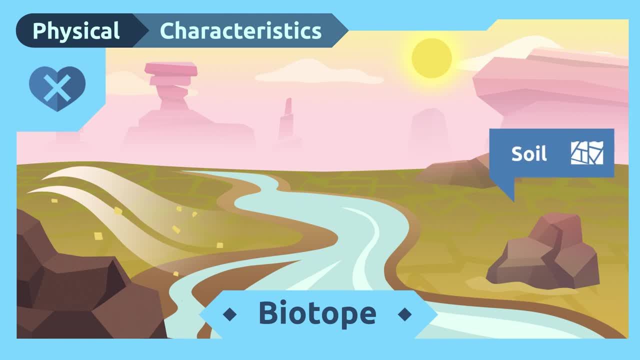 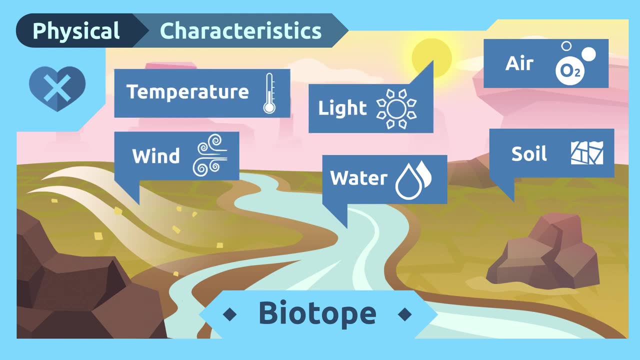 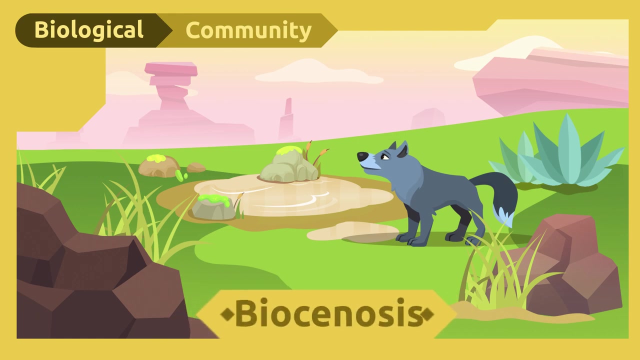 include non-living elements like the soil, the water, the air, the wind, the light or the temperature. The biological community that lives in those surroundings is called a biosynosis, That is to say, the living beings that live in a physical area, Among the living beings that. 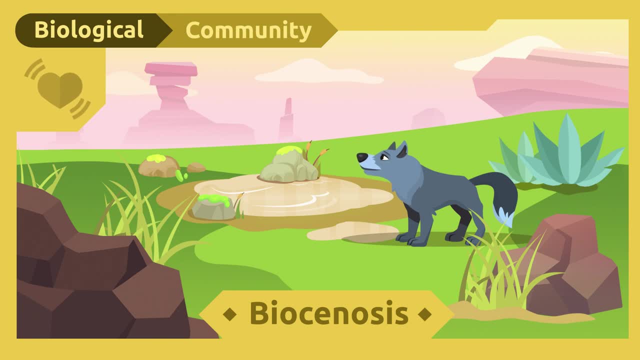 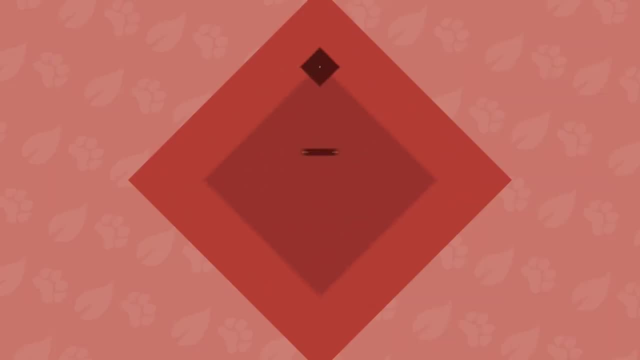 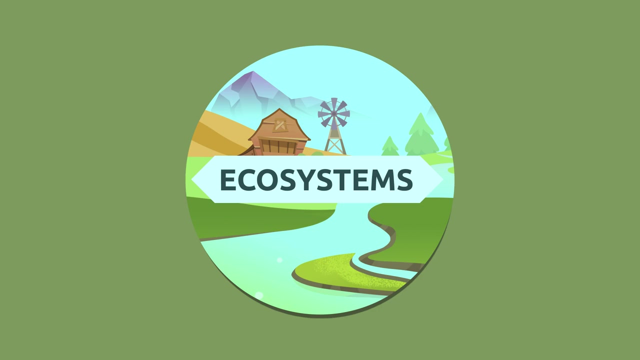 make up the communities in an ecosystem. we can find microorganisms, plants and animals. In one example, we found a Hallucination. What's what? in a biosynosis IDEALS, We distinguish between two types of ecosystems: Natural ecosystems and Artificial ecosystems. 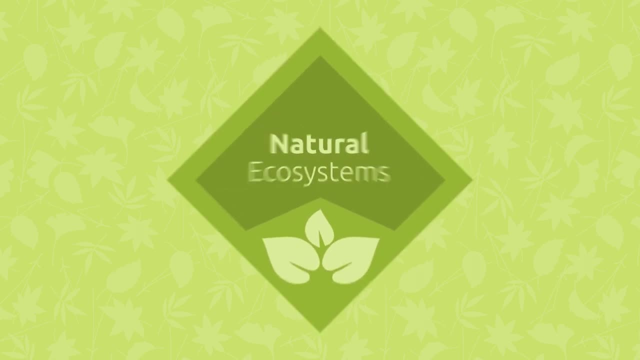 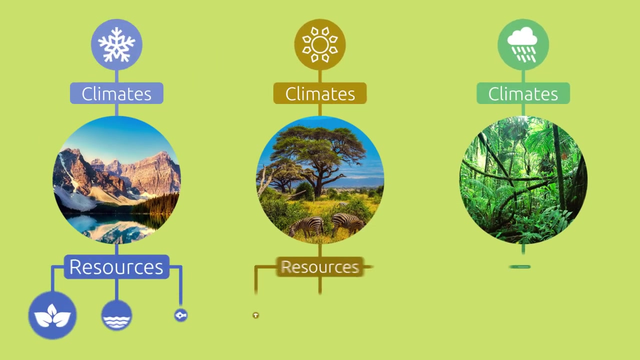 What are Natural ecosystems and artificial ecosystems? Natural ecosystems are those areas that have developed without human interventionіє- cabcar2- Where consciousness can liberation and reanimation in the complexities of an ecosystem. Natural ecosystem diversity occurs due to different climates and resources found in 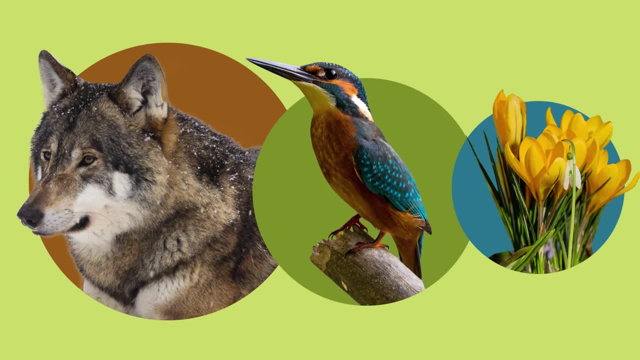 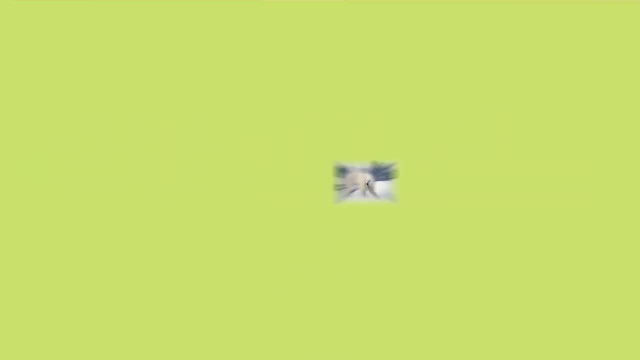 every one of them because, according to natural ecosystems, there isO. so every one weird living there. Grandma said: where there is animal and plants and a natural ecosystem, there is, there is an original human system. Generally, Fedor 밍 developed a series of adaptations related to the environment in which they live. 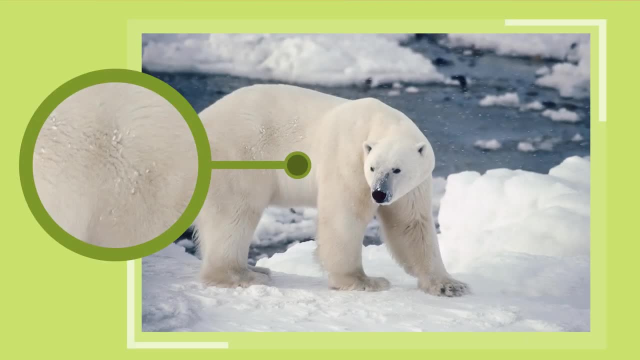 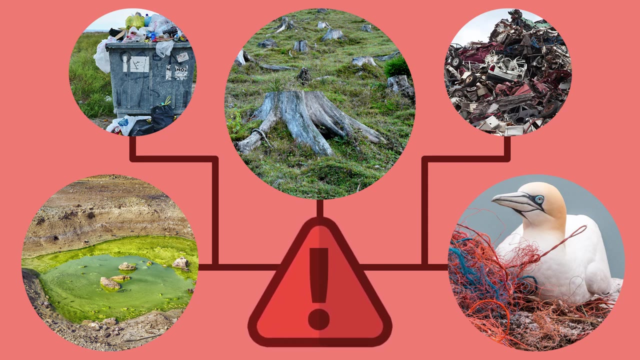 Polar bears, for example, are white to camouflage themselves in the North Pole environment. If those environments are destroyed or if there's a change in the resources, the interaction among the elements of the ecosystem would be altered, and this could endanger their existence.